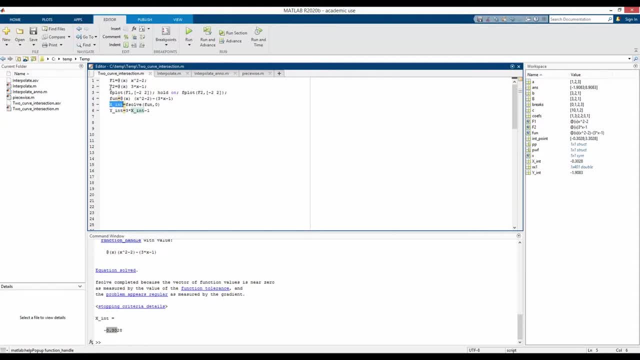 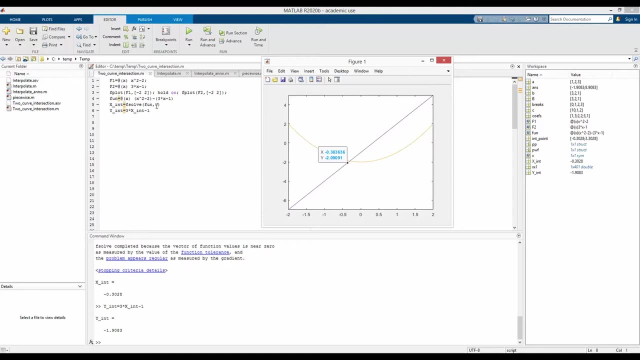 into any of these equations. So let's choose the linear equation f2, and that would give the y coordinate of the intersection point to be minus 1.09, which is somewhere approximately here. Here, within fsolve function, we have defined an initial guess for the x coordinate of this. 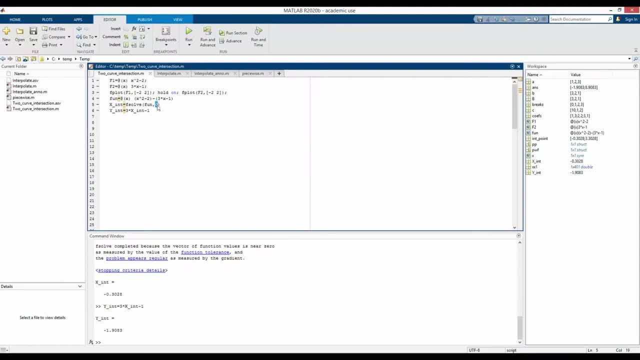 intersection point and the guess was 0 and as a result, we have got the x and y coordinate of the intersection point, such as here. But let's expand this plot beyond the range of minus 2 and and see if we have more than one intersection point. So if we evaluate that, 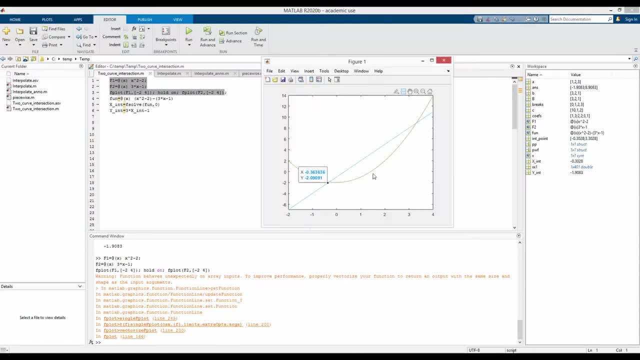 we would see beyond that point. actually, we have another intersection point somewhere between x value of 3 and 4.. So as we have our first guess close to this intersection point, because our guess was 0, so the intersection coordinate was given as the coordinate of this point. 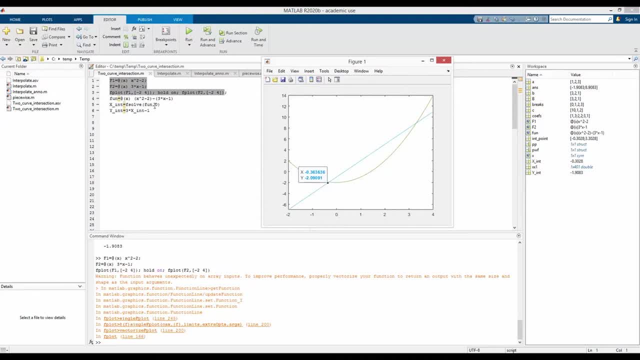 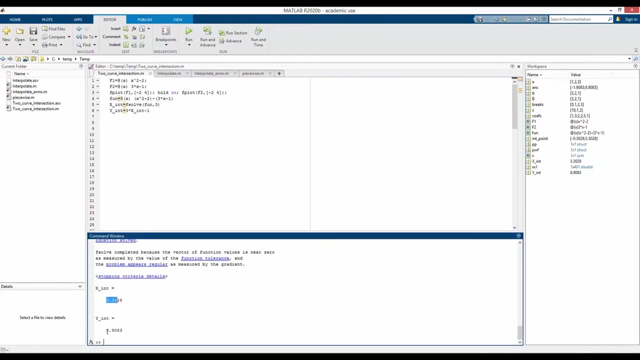 But instead let's say we start our first guess of this fsolve function to be 3, then we should get the coordinate of this particular point, which is around 3.22, x coordinate and the y coordinate 8.97.. So let's do that: We type in 3 and, yes, we have got the x coordinate to be 3.30 and y coordinate. 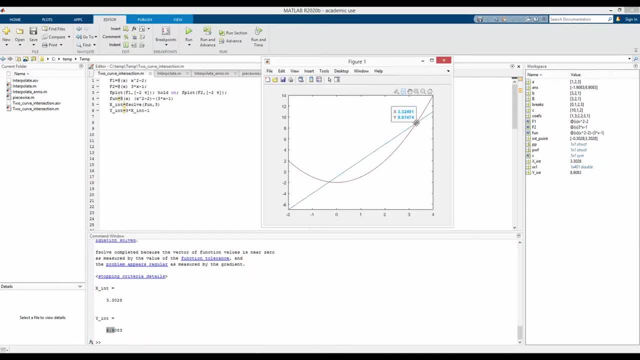 to be 8.9, as we can see in this plot. In case you have only one intersection point, then fsolve already solves your problem. But fsolve has one advantage For other method. for example, there is another function, solve, that can do the same trick, but fsolve. 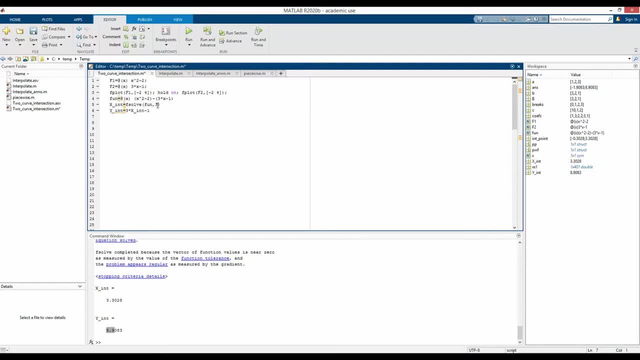 is very flexible: Instead of your initial guess to be 3, if we say the initial guess is 30, this function will still get us the second intersection point Now, if we define our function f1 and f2- same function as previous, but this time, instead of making it an anonymous function, 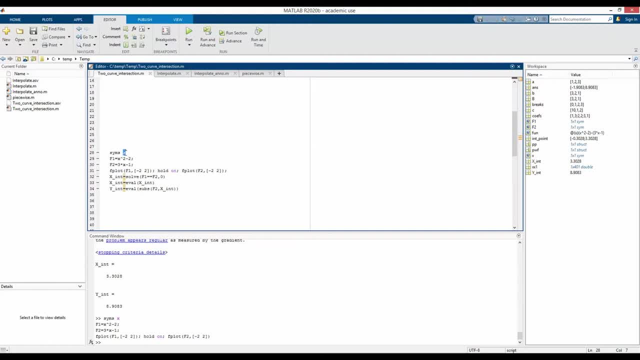 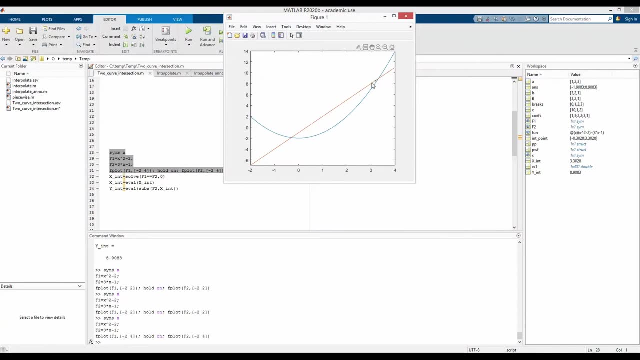 we have made it a symbolic function of variable x, So the same function. we can see it from the plot. Of course, we can expand this range up to 4 and we can see there are two intersection points. This time, as we are defining symbolic function, we can use this function solve to say that these two 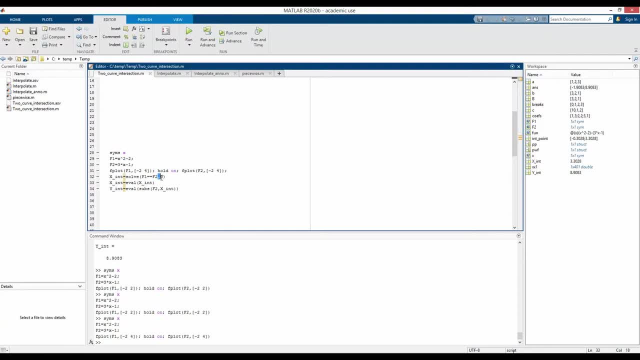 intersection points are equal and as well as provide the function solve with the initial guess- In my case I have defined it to be 0- and just by doing that, solve will solve these two functions and find both of the intersection points. So let's see how it goes. So these are the two. 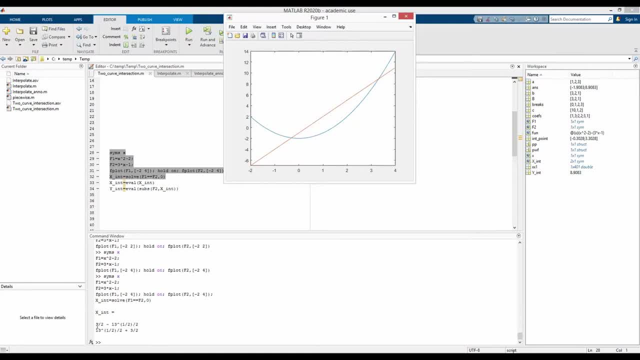 intersection points. One is this and another one this. They need to be simplified. So one way to do that is to take the x coordinate value of this intersection point, and x coordinate value of this intersection point is. just take these two points and do evaluation of them. So now we have written. 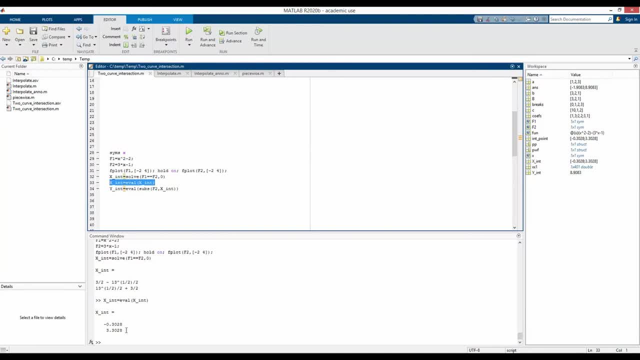 x intersection is equal to evaluation of x intersection. We get in a couple of numbers, So first intersection point is 0.3 and the next one is 3.3 and which we have already checked to be correct from here. Now to get the y intersection point. 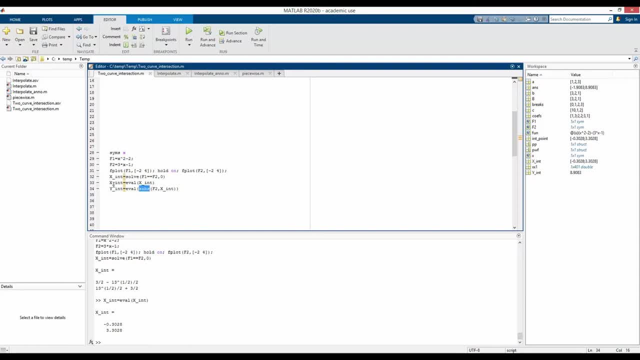 We again need to substitute the value of x intersection point in function f2.. So if we do that subs f2 in x intersection point, we will get the y coordinate of first point and the second point of intersection. We can put the whole thing and do a evaluation in the same line, such that 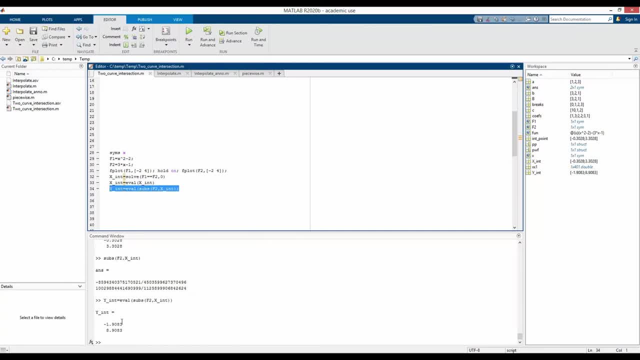 it gives y coordinate of the intersection point as a couple. One disadvantage of using solve that our first case has to be a good one. For example, if we have our first case to be 10 for solving these two equations, we would get the solution actually fails and we don't get.